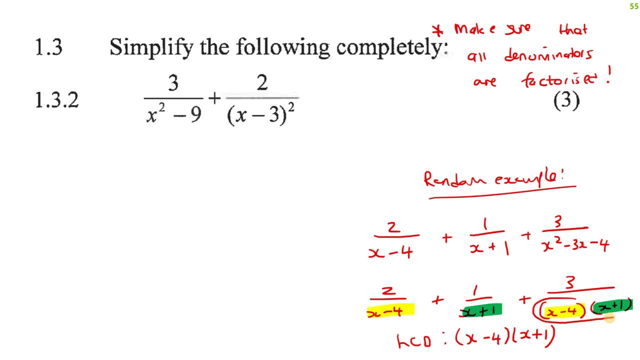 only need to be multiplied with the yellow one, And this one would not need to be multiplied by anything because it already is the common denominator. Okay, But if you only looked at it over here, you would have thought: oh, this is a complicated question because now I have to use all. 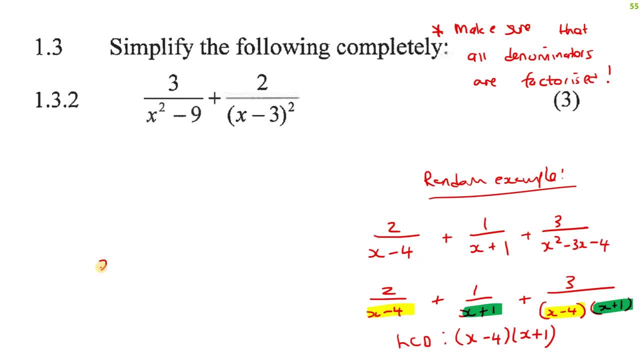 three as my common denominator, And then you might have said x minus 4,, x plus 1, and x squared minus 3x minus 4.. Because your denominator, your common denominator, and that's just going to make life really complicated. Okay, So this one here, you can't factorize this. This x minus 3, you can't do. 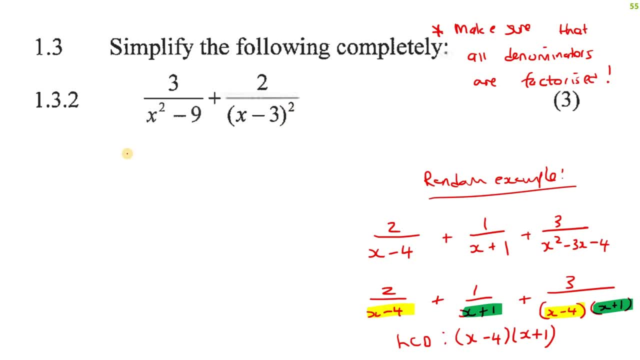 anything with that. The 2 just means that there's two brackets. So if you wanted to, we could just rewrite it as that. You could do it like that if you want. But don't go multiply this out now, because then you're going to end up with a trinomial kind of thing, And then you're just 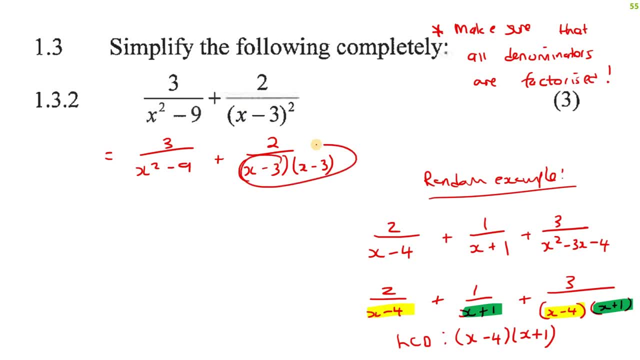 going to want to separate that into brackets anyways, So these brackets are good. Okay, This one is actually a difference of squares, right? If you factorize x squared minus 9, you can turn that into x and 3,, x and 3.. The 1s are plus, 1s are minus. That's difference of square, And so. 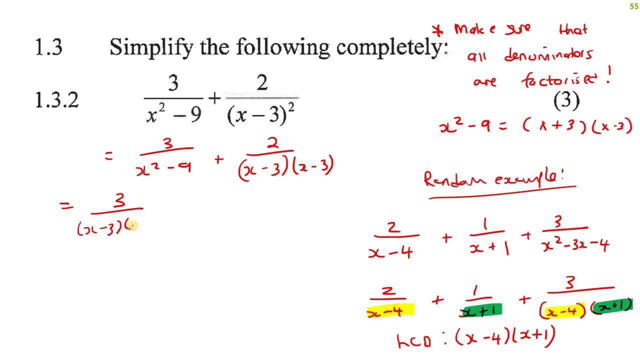 that's going to give us x take away 3,, x add 3, plus 2 over x take away 3, and x add 3.. So that's x take away 3.. Okay, So these two are the same. Then there's that one, And then there's this one. 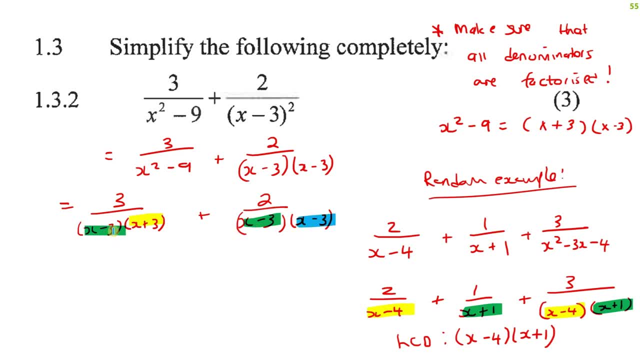 Now I know that these two are the same, but it has to go one for one. Okay, So these two matched each other, And then this one is a random, So your lowest common denominator will be all the different colors. So it'll be x, take away 3.. So we've taken care of that and that Let's not put. 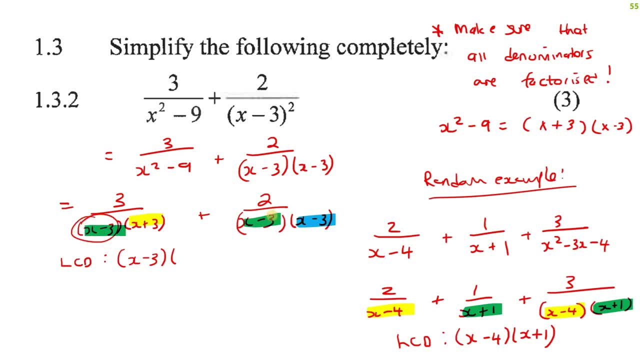 a line through it. We don't want them to think we're canceling it, But we've done this one and this one. Then we're going to do x add 3.. So we've done this one And then we're going to do this. 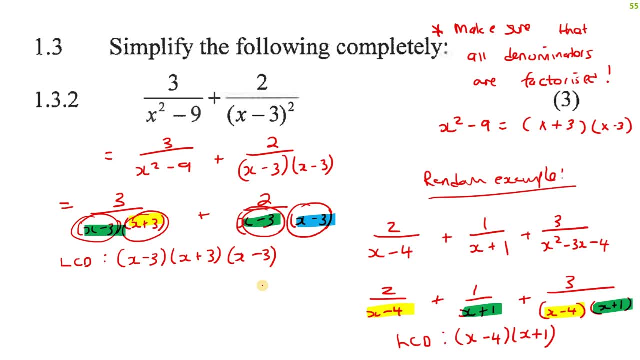 one x, take away 3.. Okay, So what this now means is that this part here still needs. well, let's, actually, let's color code these things. So the x, this x minus 3, this one will wrong color. 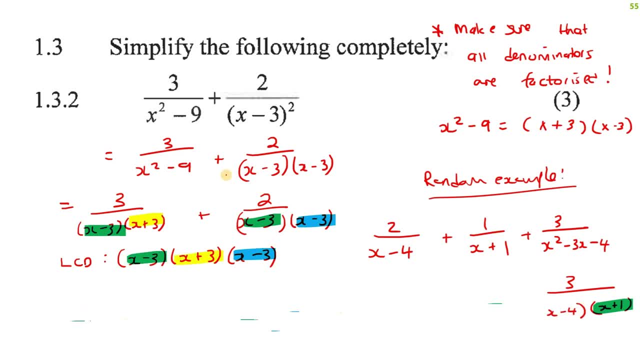 here. So the way that it now works is: we've got this common denominator, So we need to make sure that this one will end up looking like that And this one must also end up looking like that. So, if you look at this first part, what is it missing? It's missing a blue one. 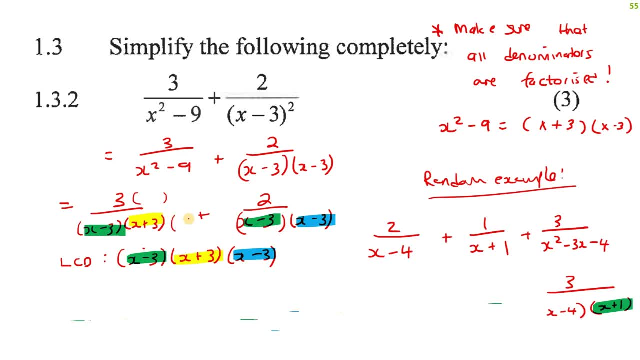 So we will give it a blue one. We'll put a blue one at the top and a blue one at the bottom, because what you do to the bottom, you do to the top. So that's going to go like this: Okay, so we're going to give it the x minus 3, which is blue, And then at the bottom, 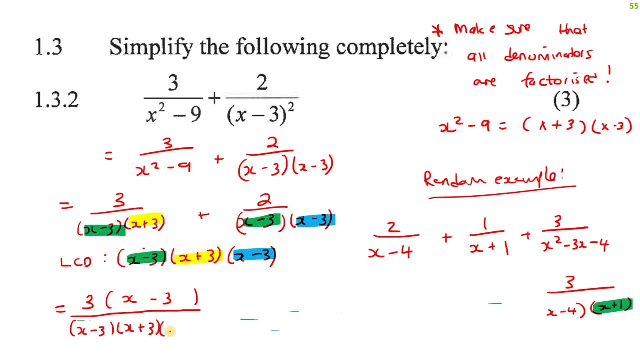 it already has an x minus 3,. it already has an x plus 3, and then we'll give it another x minus 3.. So this x plus 3 was already there, This x minus 3 was already there, And then we gave it the blue and the blue. So can you see that it's denominator? 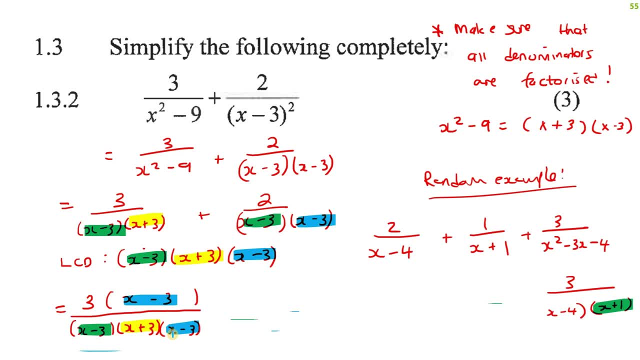 now has the different parts: it's green, the yellow and the blue. Now we're going to make sure that this one has the same denominator as this. So can you see that it's missing a yellow? So we will give it a yellow. we'll give it a yellow at the top And then at the bottom. 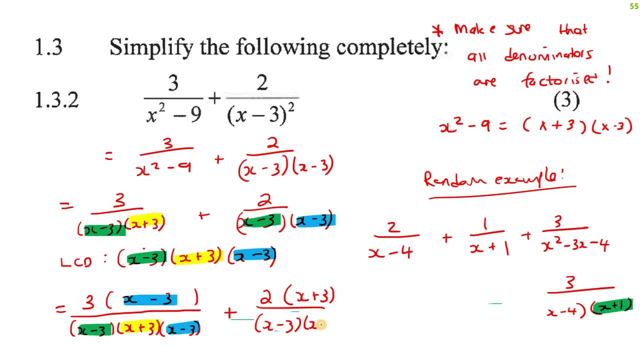 it already had x minus 3,. it already had another x minus 3.. And now we're going to give it x plus 3.. So it already had this x minus 3.. And then x plus 3,, x plus 3.. And then x minus 3.. 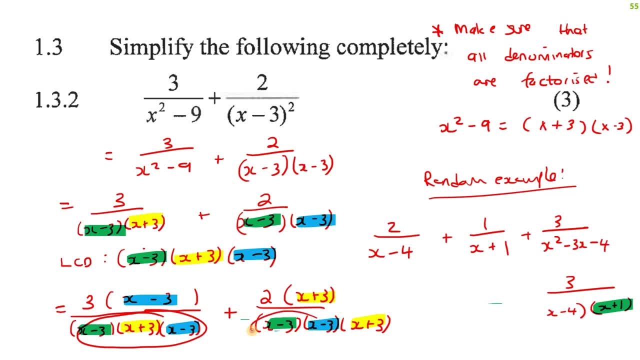 So can you see that both of these denominators now have all of the different parts of the LCD. Now what we do is, because these denominators are now the same, we can put everything together over one denominator. So, and then you're just going to go right: this part and this part, So.